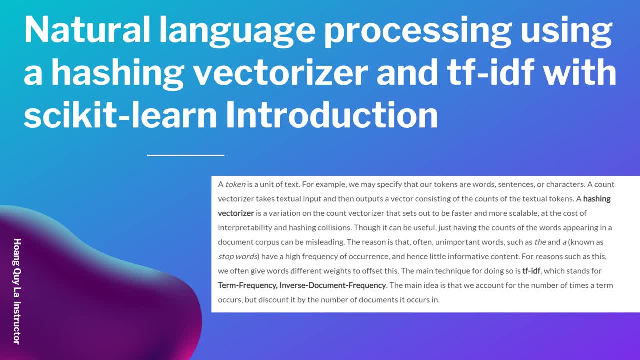 So a hashing vectorizer is a variation on the cow vectorizer that sets out to be faster. The cow vectorizer will be faster and more scalable At the cost of interpretability and hashing collisions. it can be useful Just having the cows of the words appearing in a document. code bus can be misleading. 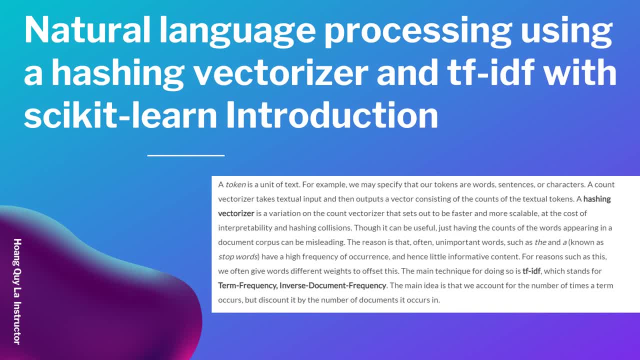 The reason is that often unimportant words such as the and a the cow vectorizer will be misleading and the cow vectorizer will be misleaded. The reason is that often unimportant words such as the and a, known as stop words, have a high frequency of occurrence and hence little informative content. 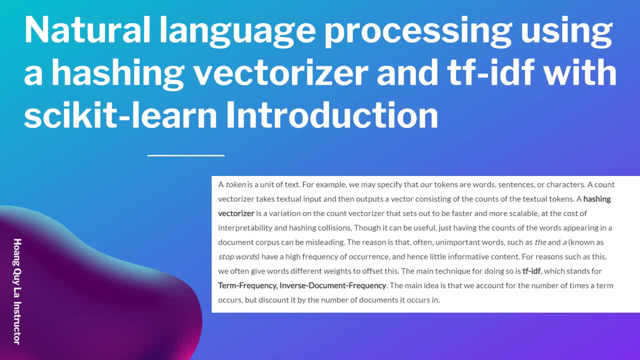 for reasons such as this, we often give words different ways to offset this. the main technique for doing so is tf, idf, which stands for term frequency, inverse document frequency. so the main idea is that we count for the number of times a term occurs, but discount it by the number. 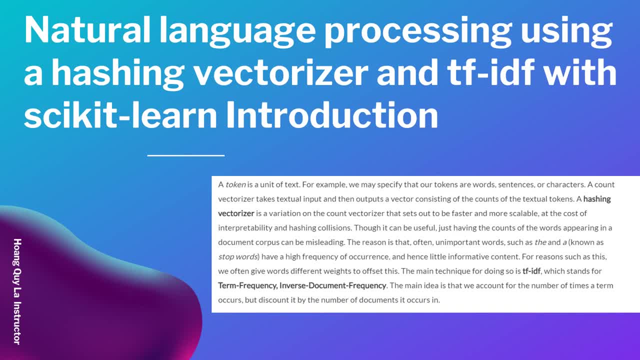 of documents it occurs in. so, in cyber security, text data is omnipresent, even logs, current conversational transcript and list of function names are just a few examples. consequently, it is essential to be able to work with such data, something you will learn in this video and the next video. so we'll implement it, and that is. 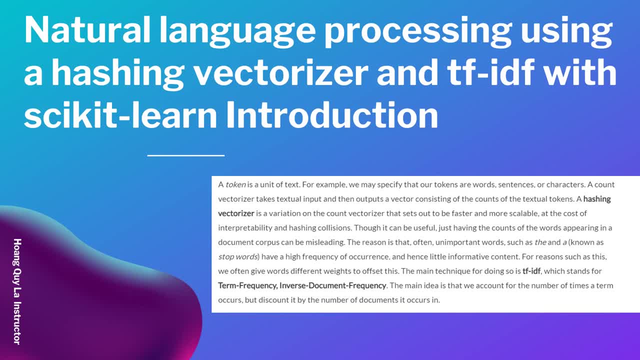 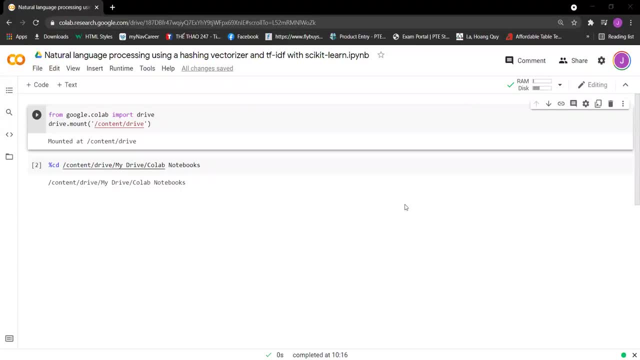 all in this video, so I hope you enjoy it and I will see you in the next video. hi, let's continue with our session. this video will implement the natural language processing using a hash vectorizer and TF-IDF with the scikit-learn. so I did mount the google drive, so I did cd the content to the. 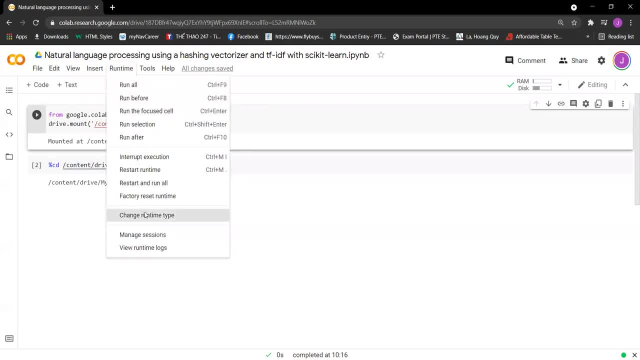 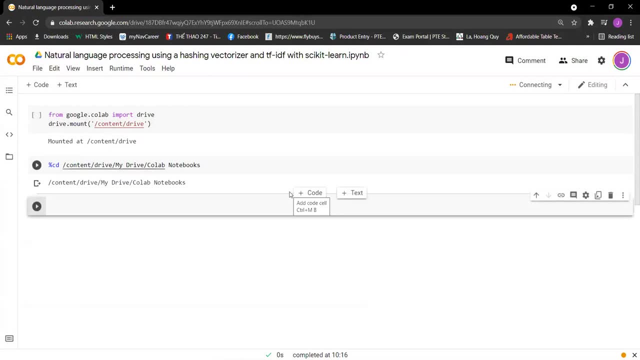 colab notebooks, and now I just change to gbzoo, so this will save our times. so now we will have the width, so let's write some nodes for that. so first we need to import this textual data set. so width open, so noNodes underscore: short dot txt. 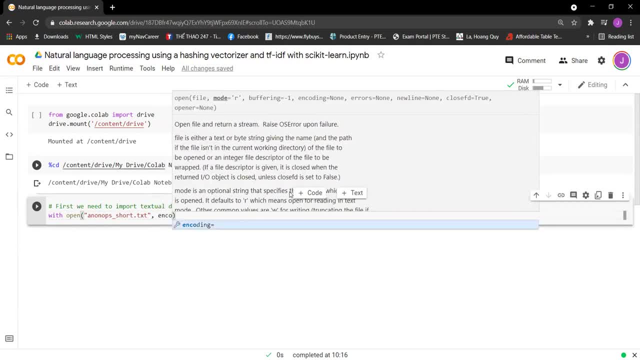 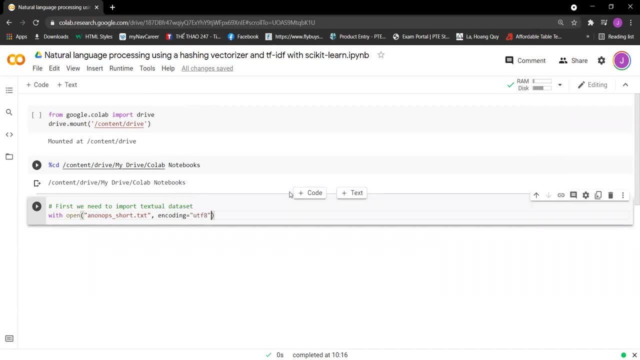 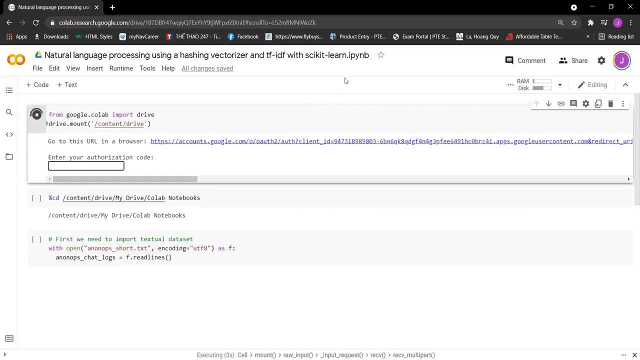 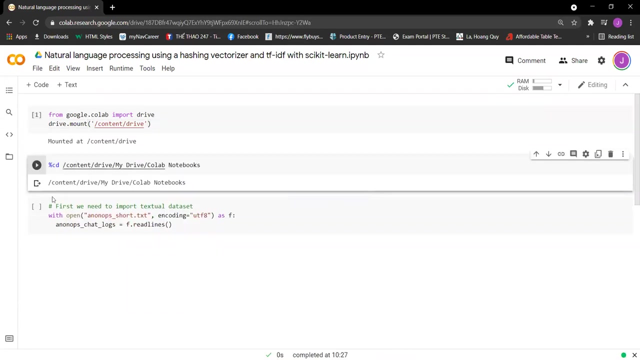 we will have the encoding, which is a UTF I as F and we have is no knobs dot underscore, chat underscore lock equal to F dot grid line. so let's run the cell. before that I need to mount drive. so I'm doing mounting drive and I will cd to the colab and then I just 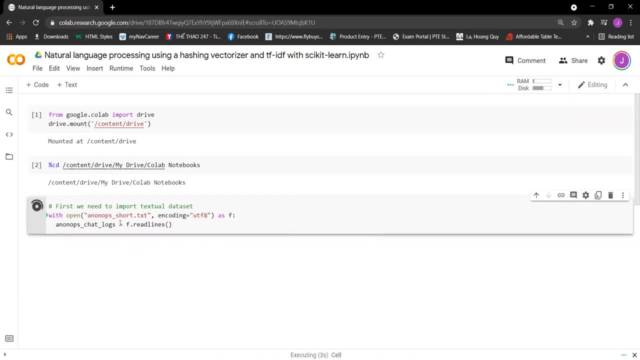 run the cell so we will open this text and read it, and it will read line by line because we have a read lines here and now. next, we will count the words in the text using the hash vectorizer and then perform writing using the CF IDF. so we will have, from SK, learn the feature. 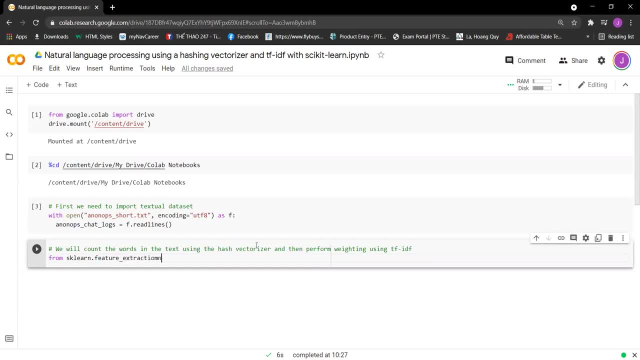 underscore instruction dot X, and we will import a hash vectorizer vectorizer, vectorizer riser. so we just copy this one and then sklearnfeatureExtractiontext will import a tfidftransformer. so now let's run the cell. so we don't have any errors. that is good, so we will write my vector equal. 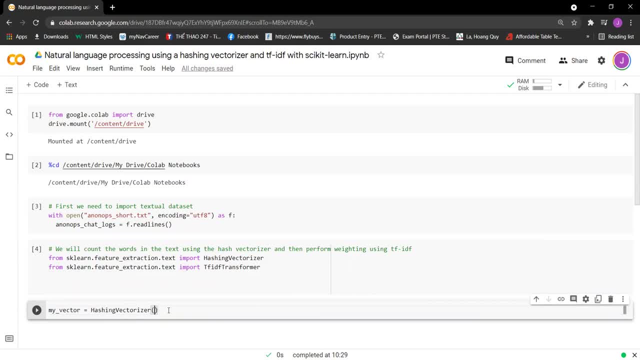 height clashing vector. so we have a input equal content. and then we got comma n: gram range is equal to 1 comma 2. and then we got x- underscore trend underscore count. and then we got x- underscore trend underscore count. and then we got x- underscore trend underscore count is equal to my underscore vector, not fit. 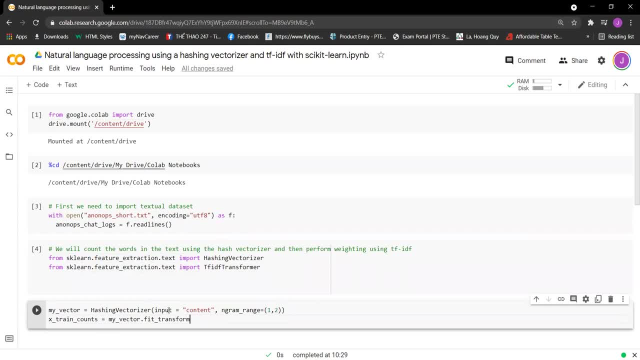 is equal to my underscore vector, not fit. is equal to my underscore vector, not fit underscore transform. so we have: is no underscore transform, so we have. is no underscore transform. so we have is no knobs, just locks, come on, and then we have. knobs, just locks, come on, and then we have. 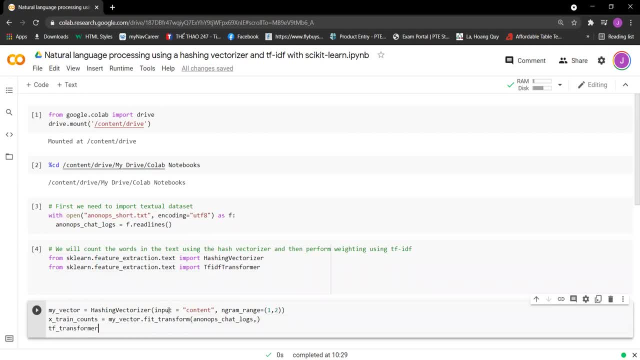 tf underscore transformer equal to tf idf transformer, and then we have is use underscore id f equal, true and finally comma, and then it will be dot, it will be dot fit. we have a x underscore trend underscore cows, and then we'll have is x underscore trend underscore tf. 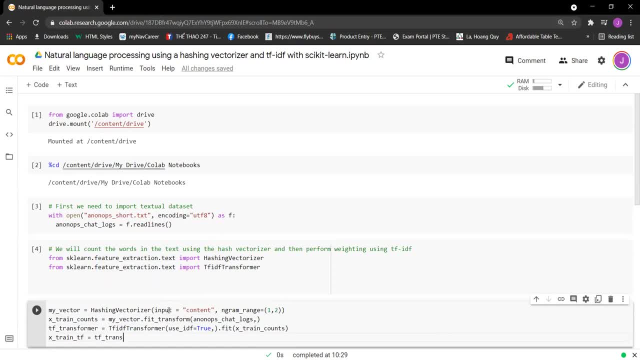 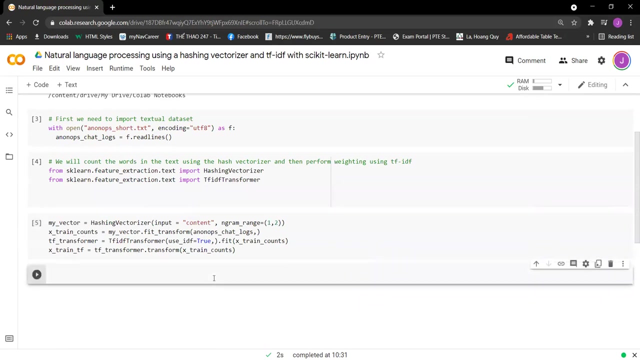 is equal to tf, underscore transformer, dot transform, transform, transform. and now we have x underscore trend, underscore cows. so now let's run the cell to check if we have any errors. and we don't have any errors. and now we have is the end result. and now we have is the end result. 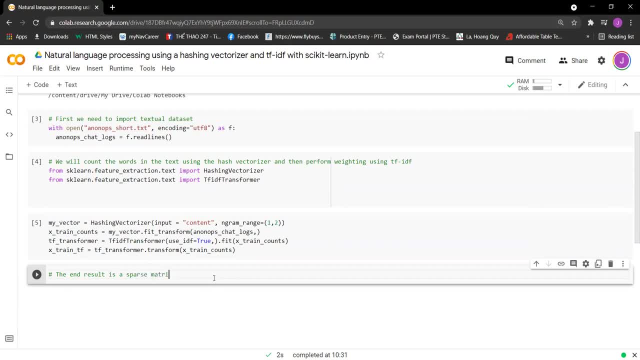 is a spa matrix, is a spa matrix with with each row being, each row being a vector representing a vector representing one of the taxes, one of the taxes. so we have is x underscore trend. so we have is x underscore trend: tf plus 1 plus 1. 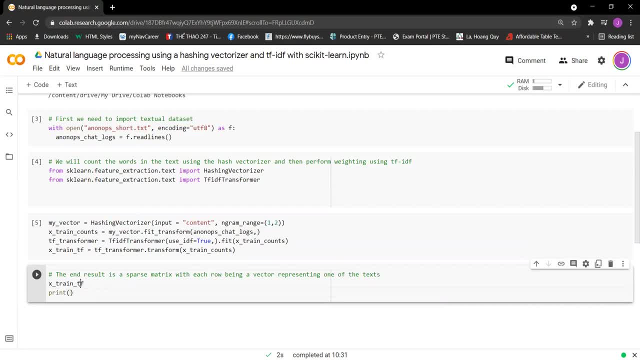 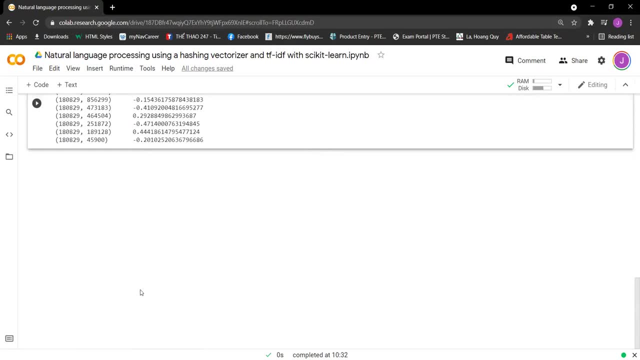 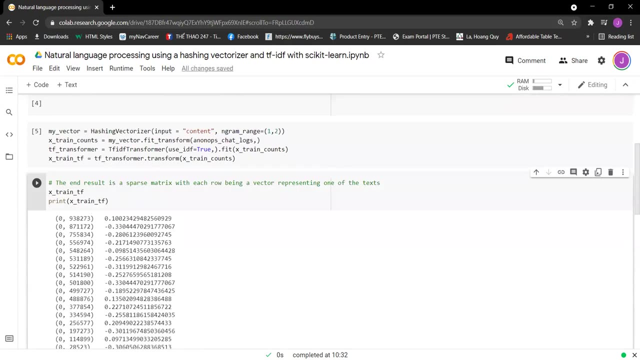 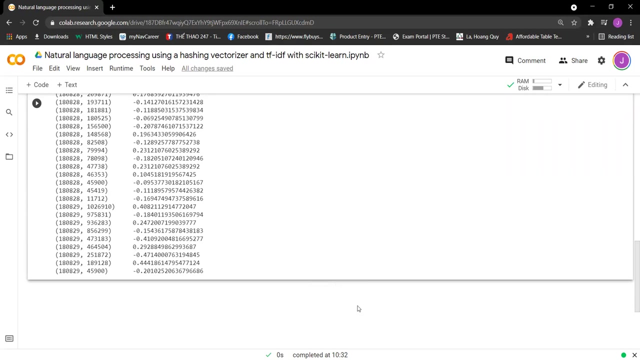 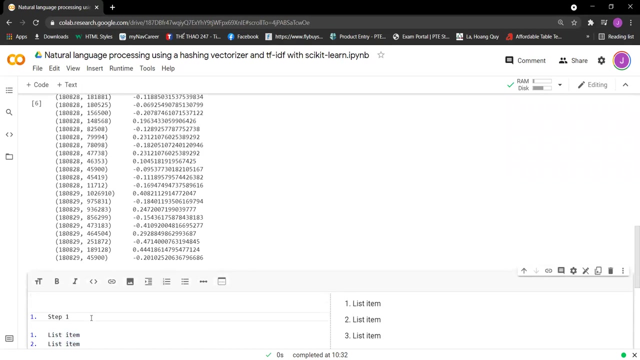 we have irons, yes, and here is one index. it's bigger than the first one. it would project and then we'll bring it, and then we'll bring it. This is the output that we will get, so we will explain how does it work. so in step 1, we load the dataset. so of course, it will be easy load the dataset. 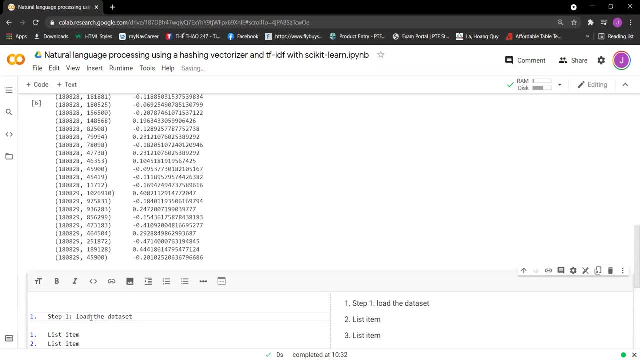 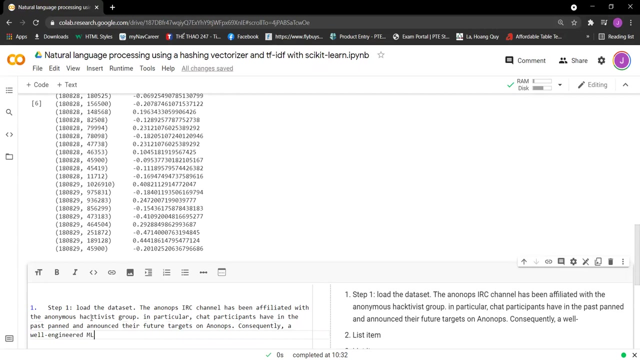 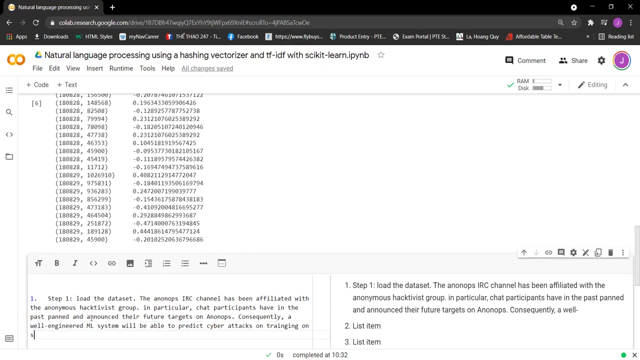 So the Anonops IRC channel has been affiliated with the Anonymous Activities group and, in particular, chat participants have been helped in the past to plan and announce their future targets on Anonops. so, consequently, a well engineered ML system will be able to predict cyber attacks on trending on such data. 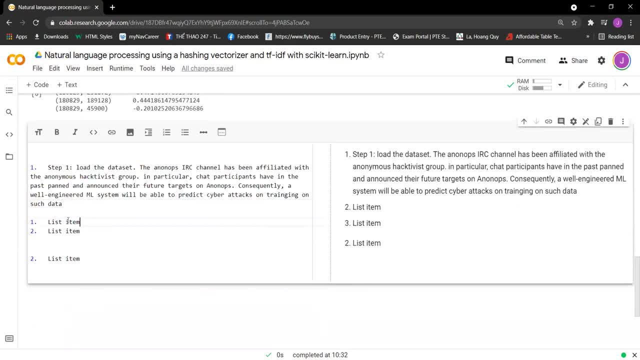 Now let's move to step 2. So step 2 is we instantiated a hashing vectorizer. So the hashing vectorizer gives us counts of the one and two grams in the text. so in other words, in other words, singleton and consecutive pairs, pairs of words. 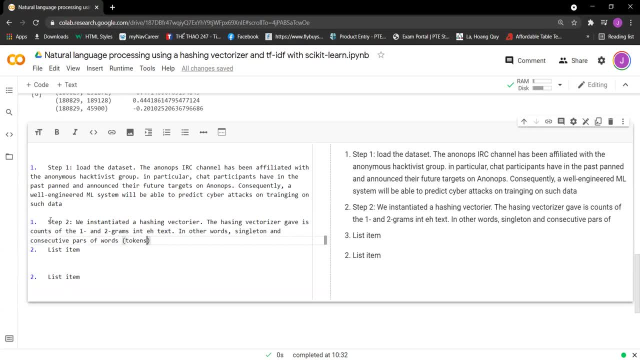 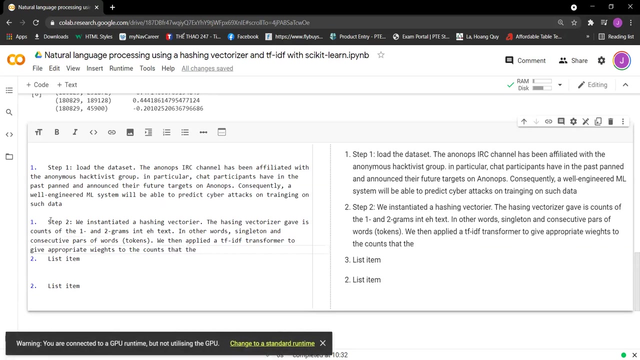 which is a token, pairs of words, which is a token. we can apply: TF, IDF, transformer to be transformer, to be appropriate, appropriate, appropriate weight. repeat: Yes, Starting withель the, the shirt of the planted plants Outside of the 世界. this, So our final result is a large bar matrix representing the occurrences of 1,, 2, and. 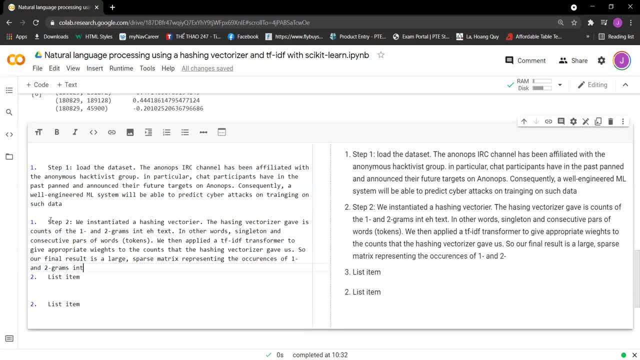 2 grams in the Texas weighted importance. So the final step- step 3, is that we did examine the front end of a bar matrix, The bar matrix representation of our features data in SkyBee. So, and that is all in this video, 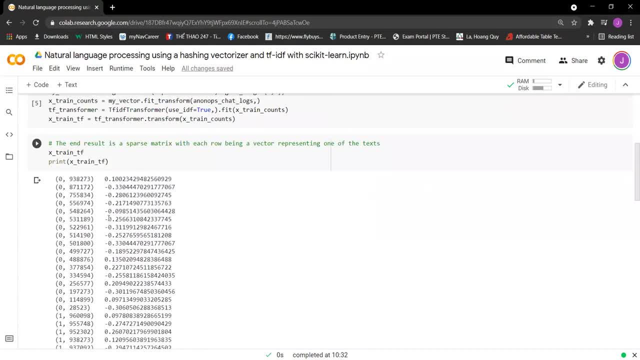 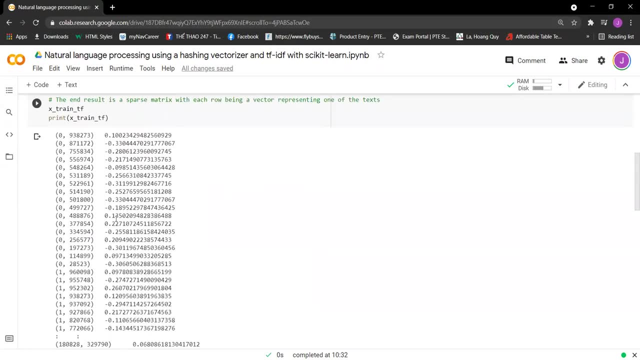 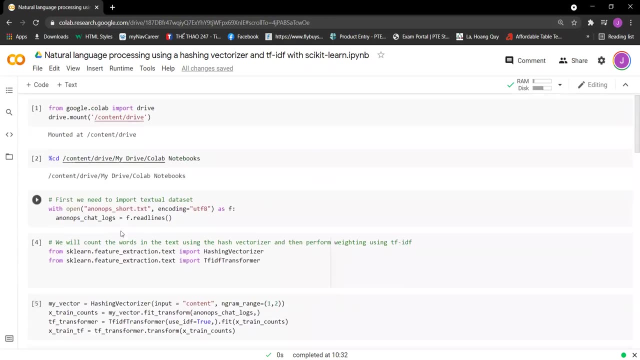 So I hope you can run successfully And get the result as same as mine. So if not, do not worry, You can check my code and then copy and paste it to see what did you go wrong. And that is all in this video and in this project. 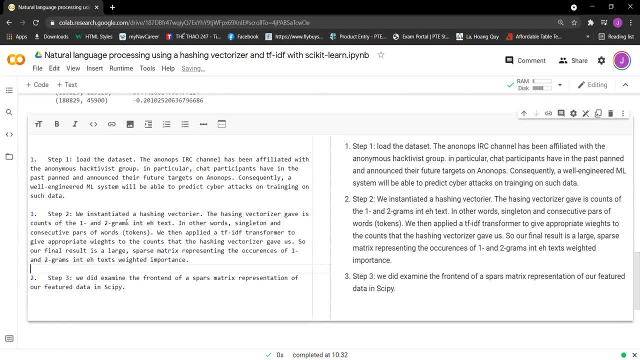 So I hope you enjoy it and you learn a lot, And I will see you in the next video.